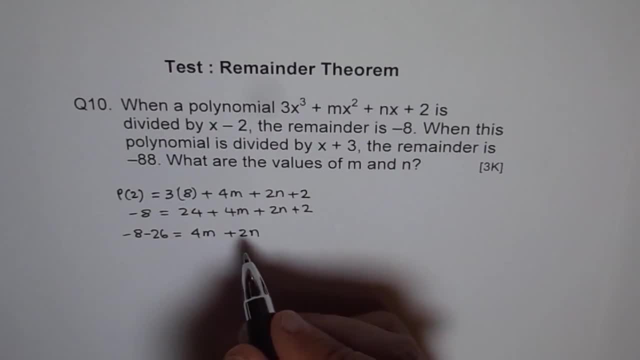 So minus 24 and minus 26 gives us: minus 34 is equal to 4m plus 2n. We can divide by 2, right. We get minus 17 equals to 2m plus n right, So that becomes our equation number 1.. Let's call this equation 1, right. Now let's try to do the other half on the right side. 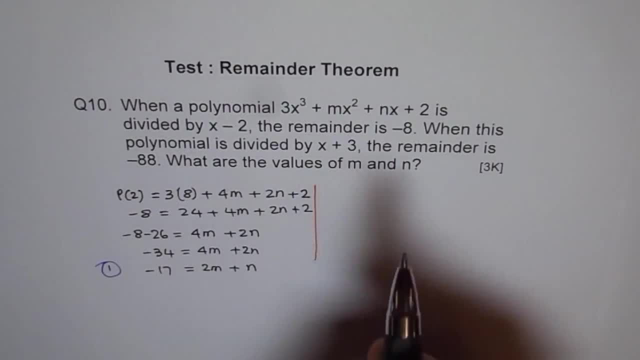 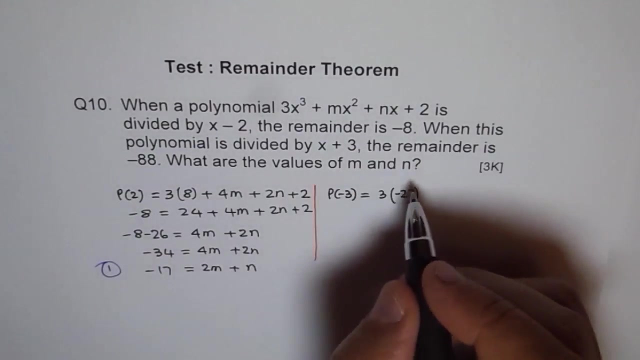 1,. this polynomial is divided by x plus 3.. That means p of minus 3, right. So we have: p of minus 3 equals to minus 88.. So let's plug in minus 3 here, So we get 3 times minus 3. cubed is minus 27,. right, And minus 3 will become square plus 9m 3, squared is 9.. Minus 3n plus 2, correct. 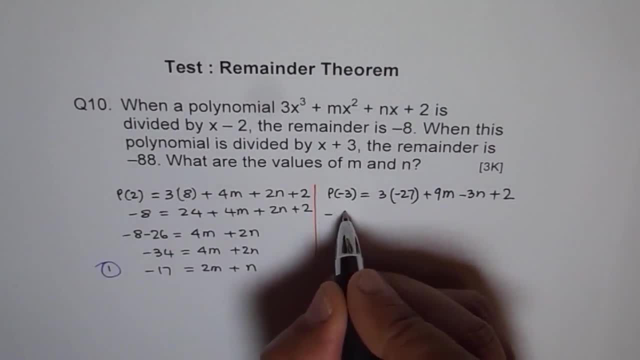 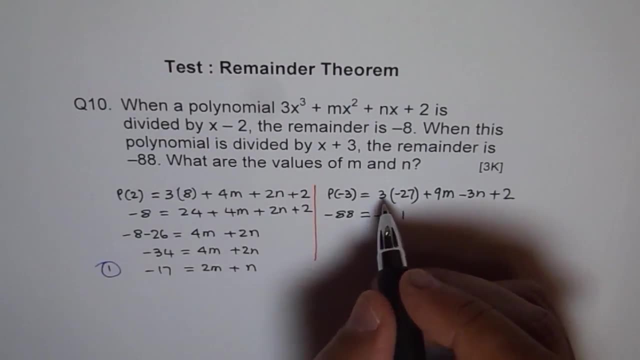 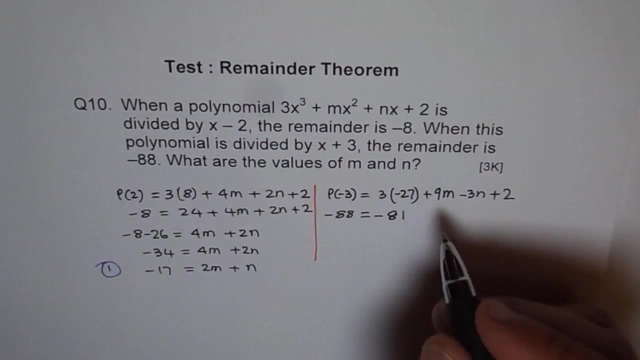 This minus 3 is minus 88. So we'll put minus 88 here equals to 3 times this, 3 times 7, 21,, 3 times 2, 6 and 81, correct. And plus 9m minus 3n plus 2, right. 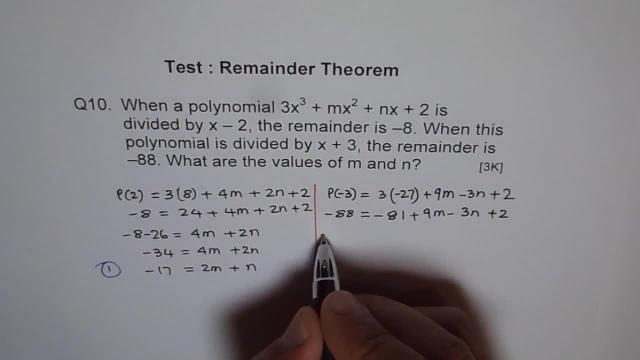 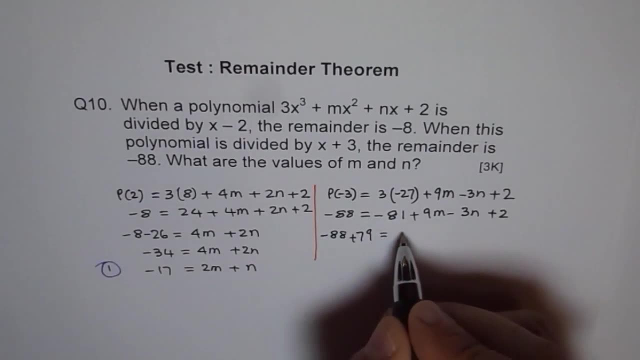 Now we'll bring these terms on that side. So we'll say minus 88. And this is plus 79 equals to 9m minus 3n, correct, Now, when you do this, so it is minus 9 equals to 9m minus 3n. We can divide by 3 this time, right? This minus 3 equals to 3m minus n. So that's what we get. 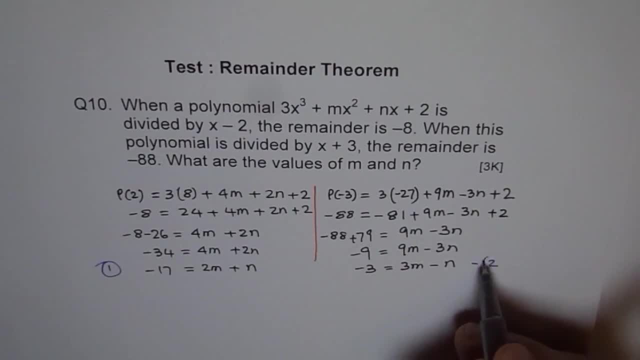 Let's call this equation 2.. Now from these two equations we can find two variables, right? So we have 3m minus n, 2m plus n. Let's add them correct. So if I add equation 1 and 2, what do I get?